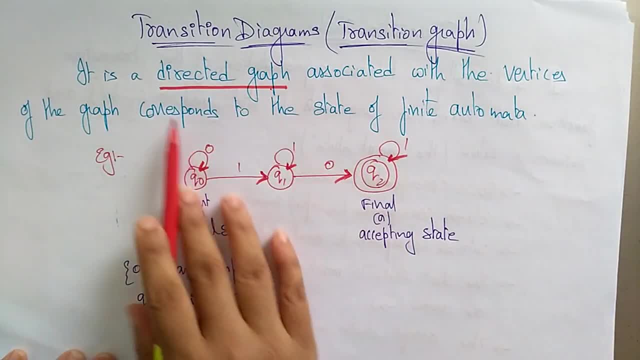 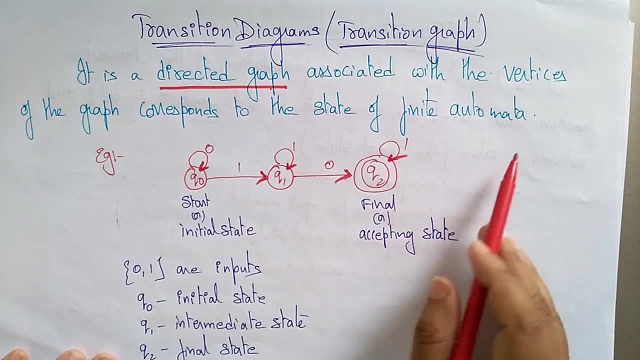 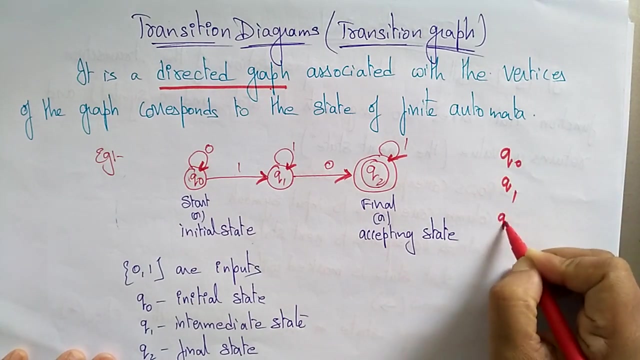 is pointing to some state. you call it as a directed graph. So it is a directed graph. associated with the vertices of the graph corresponds to the state of a finite automata. So let's take a finite automata. So here you are having three states. What are the three states? Q naught, Q1, Q2.. So these are all the three states that are present And the starting state is the Q naught is the initial state and Q2 is the final state. So whenever the final state is there, you have to. 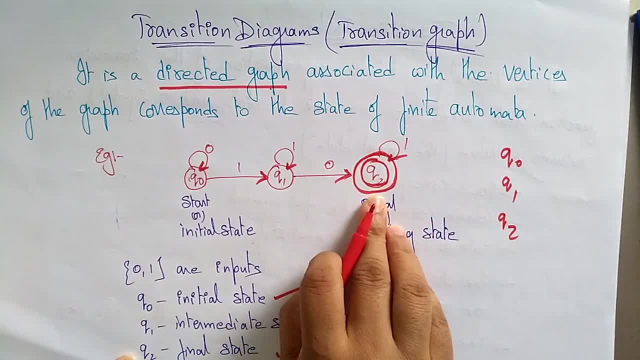 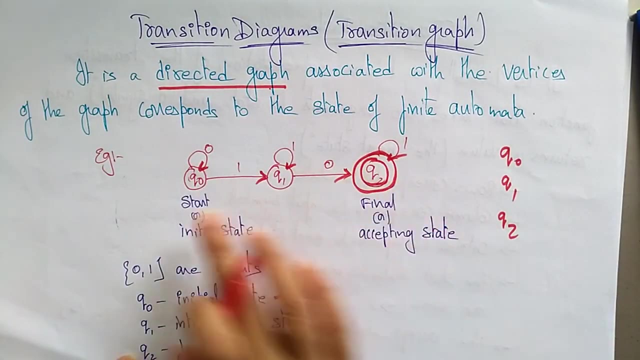 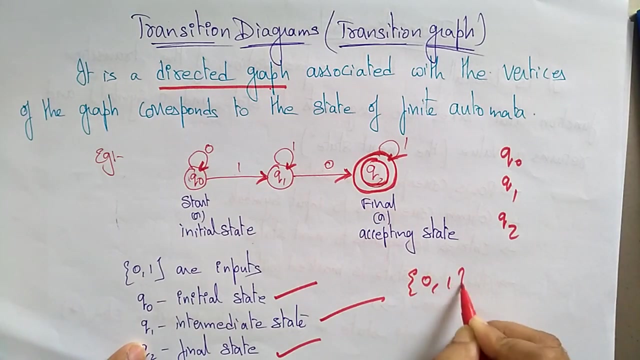 represent it with the two circles. So this represents the final state. This is the indication of the final state, or you call it as an accepting state. So Q naught is the initial state and Q2 is the final state. Whatever the states that are present in between the start and the final, initial and the final, those states, you call it as an intermediate state And here there are two inputs. We are taken 0, 1.. So 0 is the one input and 0, 1 is another input. 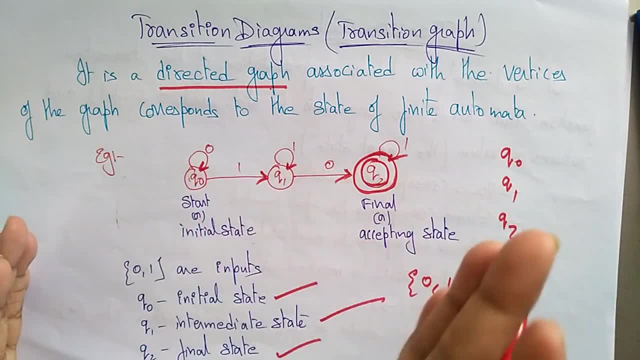 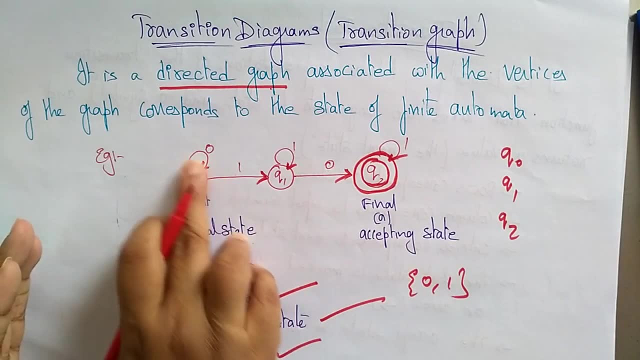 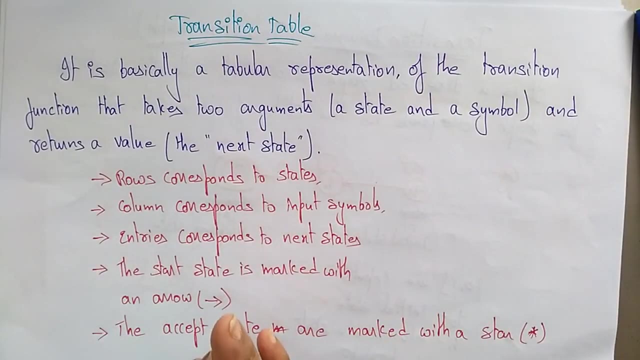 Okay, So initial state, final state, intermediate state, and this should be represented with a directed graph holding the inputs. Now let's see the transition table. A transition table here. it is basically a tabular representation Table itself. we know that we have to represent it in the form of a rows and the columns right. 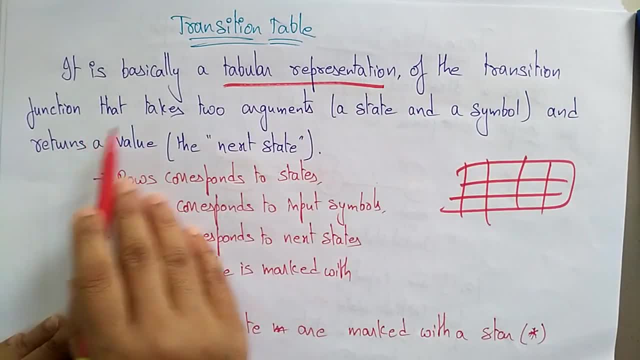 It is a tabular representation of the transition function. Okay, So we have to represent it in the form of a rows and the columns right. That takes two arguments. That is, a state and a symbol. We are taking a state and a symbol. 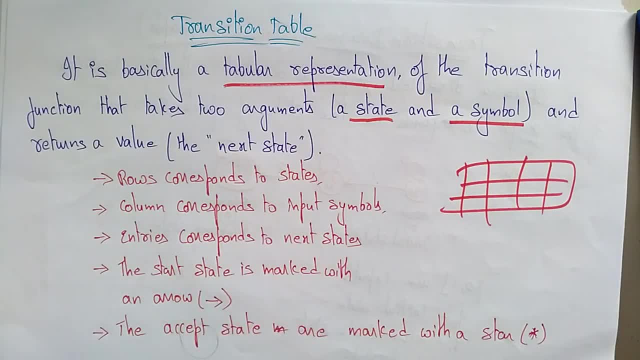 State means either initial state, intermediate state for final states, And the symbols are nothing but the input symbols. Here. in this previous example, the 0 and 1 are the symbols And the written value is nothing but the next value. That is a transition function. You know that. 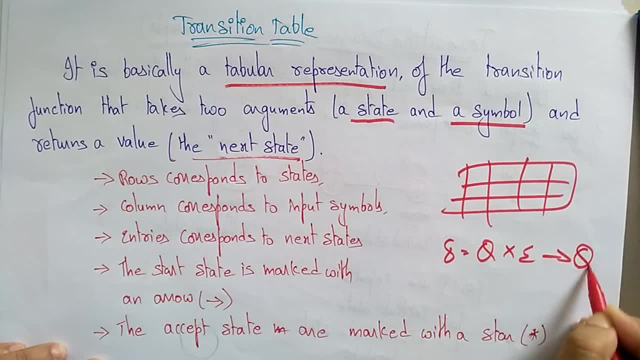 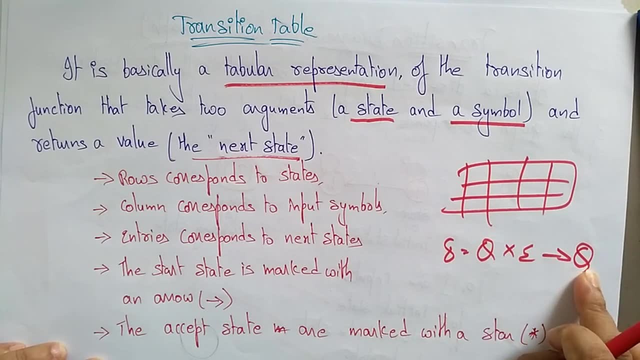 delta is equal to. you know, Q into sigma, you will get the Q, Okay, Initial state. some state, not the initial state. Symbol is equal to future state. Symbol is equal to future state. you will get the next state. so that you have to know. now let's see the transition table, the. 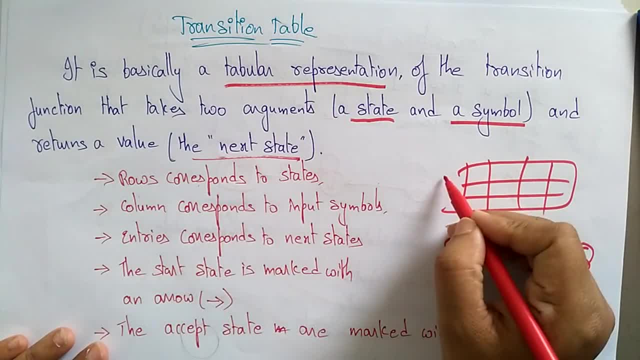 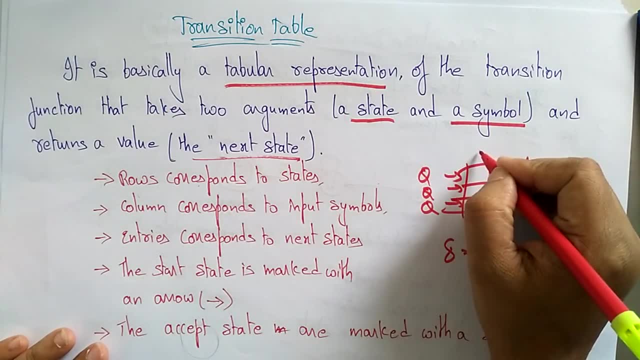 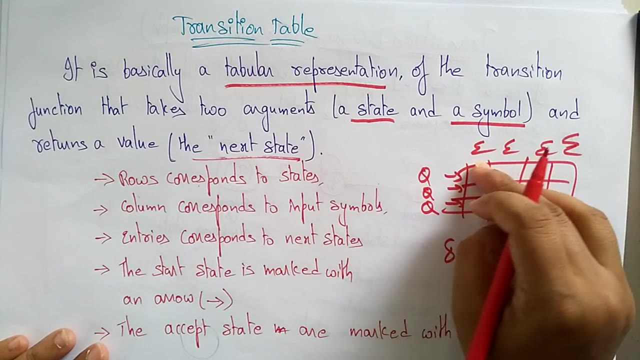 transition table consisting of the rows corresponds to the states. the rows are represented with the states. okay, so the rows are represented with the states and the columns are represented with the input symbols. input symbols, that is 0 or 1 or whatever, maybe a, b alphabets. so set of strings. 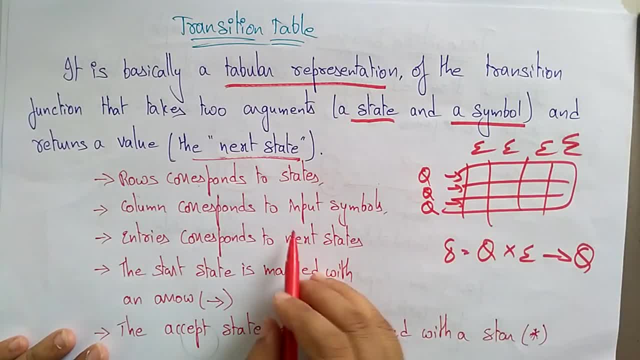 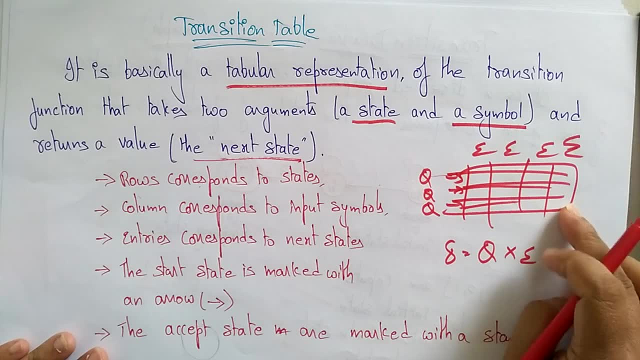 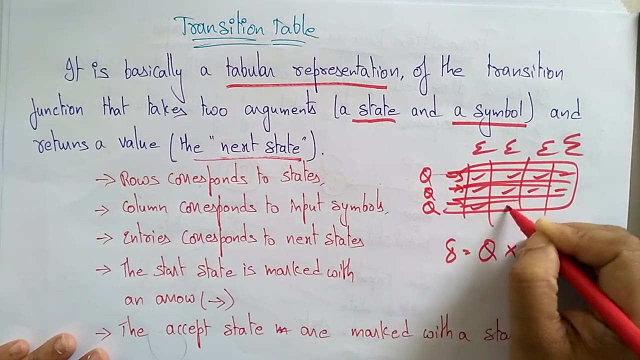 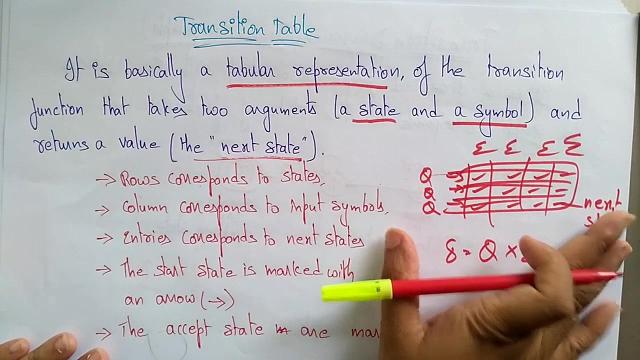 so set of symbols, that is alphabet. so rows represents the states and columns represents the input symbols and entire corresponds to the entries. so whatever the entries that are present, so entries, these entries- represents the next state. remember that whenever you are writing the table, the rows represents the states, column represents the input symbols. 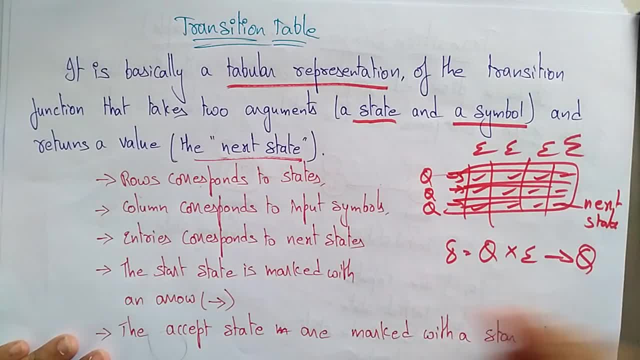 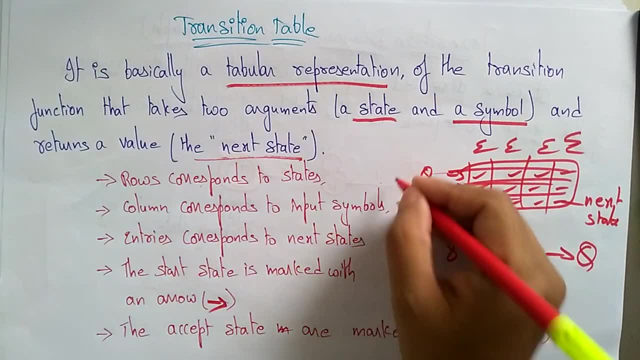 and the entries represent the next state. so these entries represent the next state and the entries in that state should be the next state. the start state is marked with an arrow. okay, so start states always marked with a. suppose this is a start state, you have to mark it with. 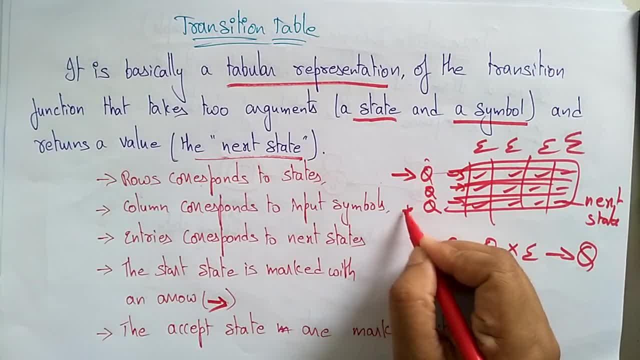 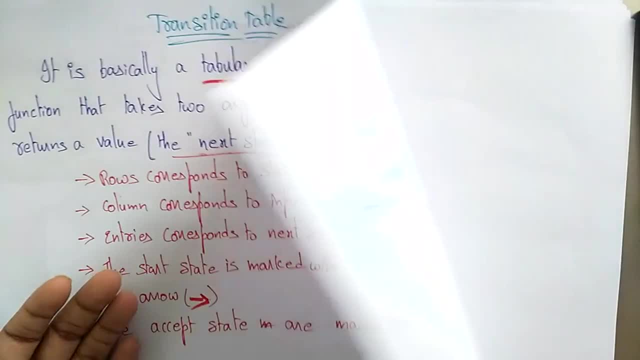 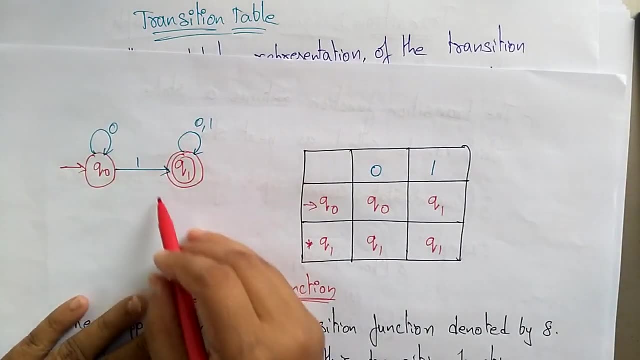 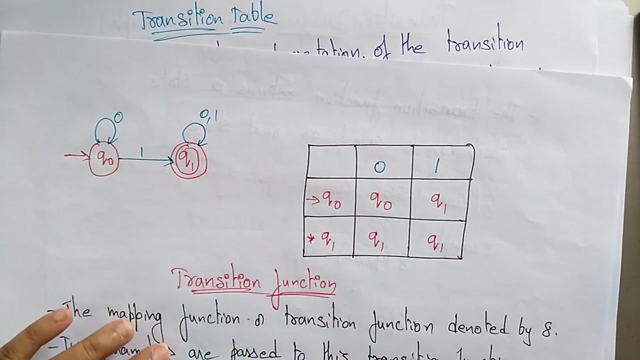 arrow and acceptance state. the final state should be marked with star. remember that. these are the points that you have to remember why while you're implementing the table. okay, so let me show you, show you, how to draw the table. let me take this transition diagram. by seeing the diagram, i have to draw the table. so q naught q1. these are the two states. 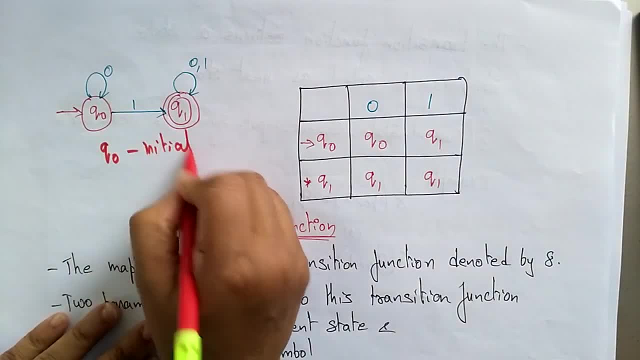 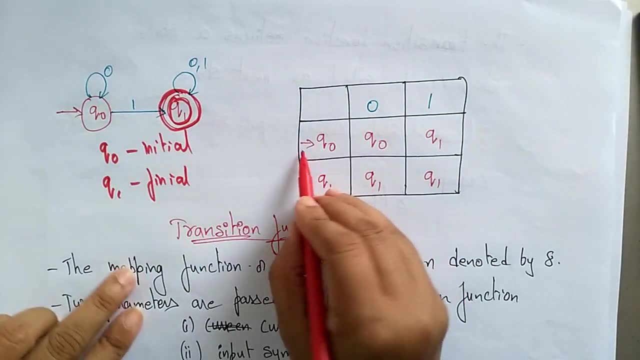 so q naught is the initial state and here i have taken only two states and q1 is the final state. so the final state always represent with two circles okay and the q naught. here, uh, in the rows you need to write the states q naught and q1 and in the columns you have to write: 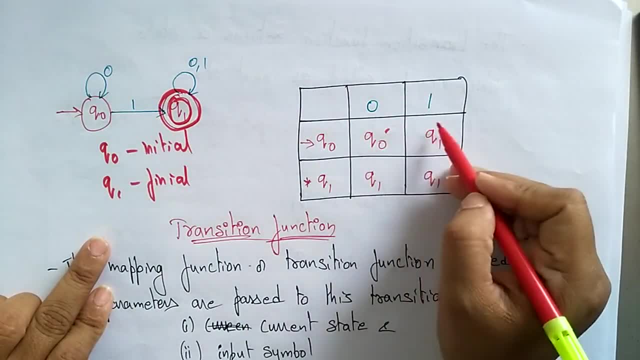 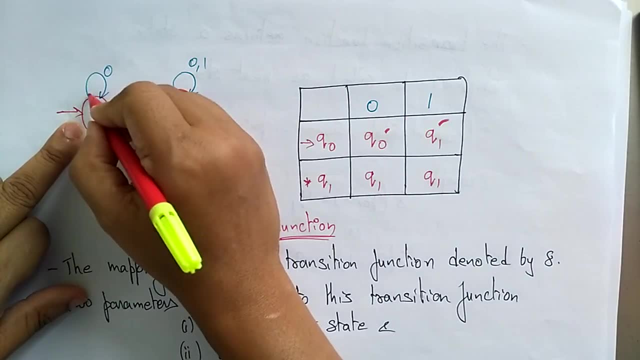 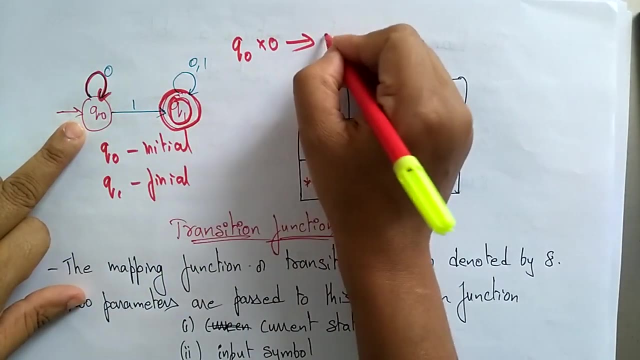 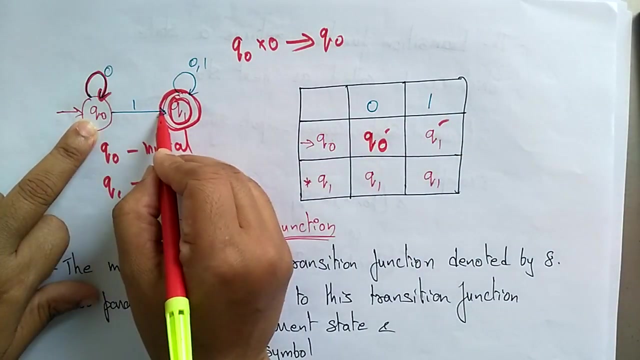 the input symbol. zero and one are the input symbol and the entry should be the next state. so now see: q0 to 0, q0 to 0. what is the next state? if q0 to the 0, it goes to the next state. what is the next state? q0 itself. so write q0 here, next q0 on 1. q0 on 1, it goes to.